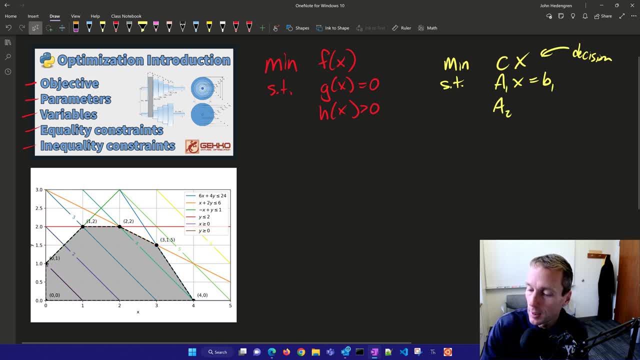 constraint, And then I could also have a2 times x and is greater than b2.. That's my inequality constraint. So let's just solve a simple problem. just to demonstrate this: So we're going to have a vector c times x of decision variables, And then I'm going to have a vector c times x of 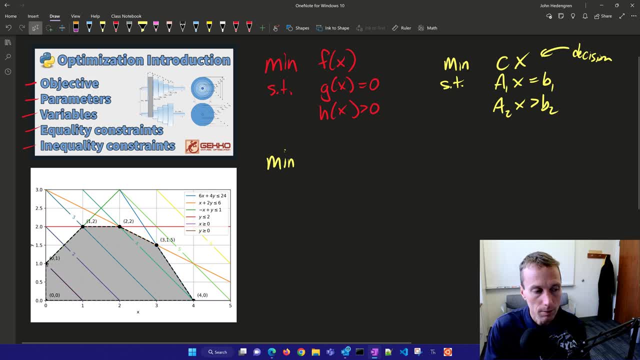 decision variables, And then I'll have an objective that's going to be minimized: 0.5 times x1 plus 0.8 times x2, plus 0.7 times x3.. And then we're going to be subject to- and this one is going to- 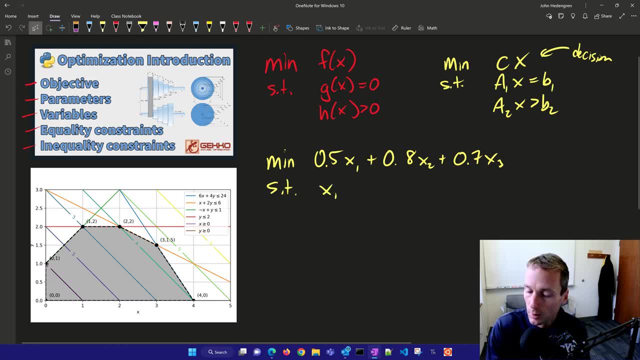 have an equality constraint and an inequality constraint. So just for the sake of simplicity here I'm going to add up x1 plus x2 plus x3. And that is going to be equal to five, And then we're going to have x2 plus x3 is going to be greater than well. actually, let's make this. 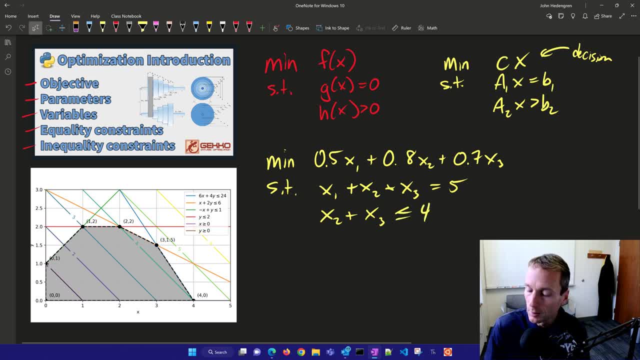 less than four. Okay, less than or equal to is equivalent when we're dealing with numerical values. Okay, so here's our optimization problem Right here that we want to solve. So let's go and set this up and solve it in Python And then 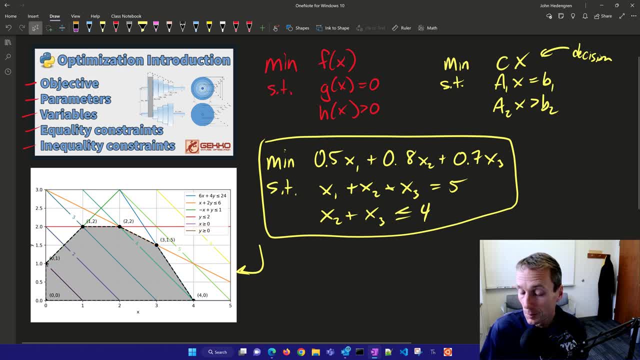 we'll move on to one that's just a similar linear programming problem, where we're going to solve this one as well, or we'll maximize x plus y. Okay, subject to those constraints, We'll do that one next, But let's go and do this simple one right here first. Okay, so let me go just move this. 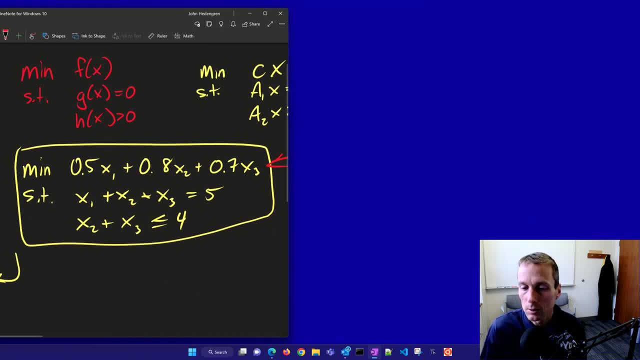 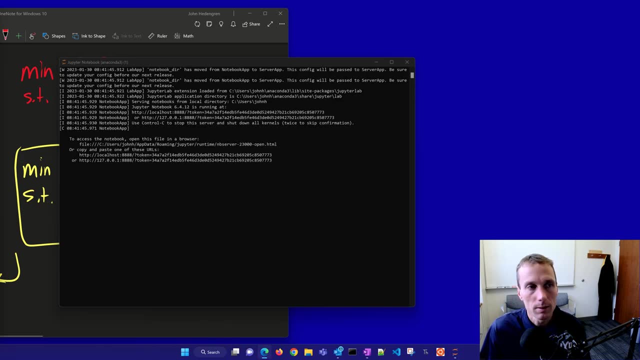 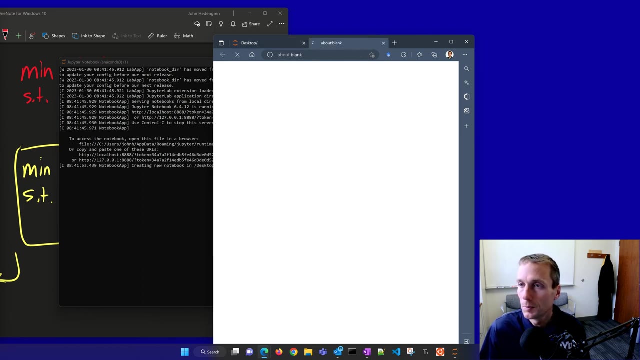 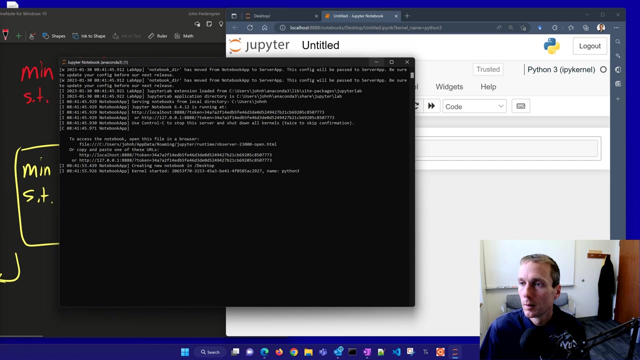 out of the way here. And then let's go and start up a Jupyter Notebook, And I'll just start this up, Okay, on my desktop, and then create a new Python three Jupyter Notebook here, Okay, so the very first thing that I'm going to do with this is 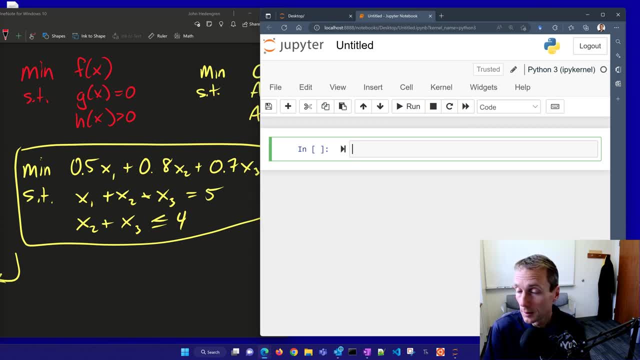 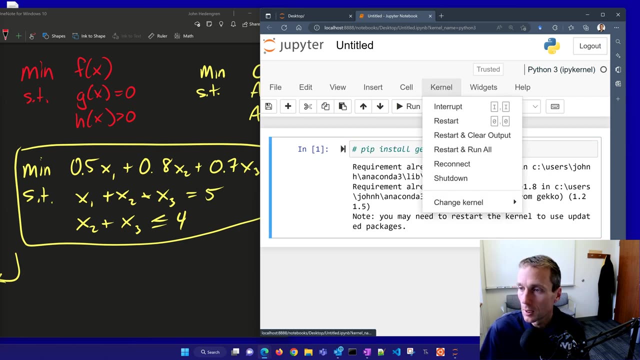 go ahead and just install a package called gecko. Okay, so that's going to be pip. install gecko. you only need to run this once And then, after you run it, then you can comment it out. And if it just installed, then just come here to kernel and restart. 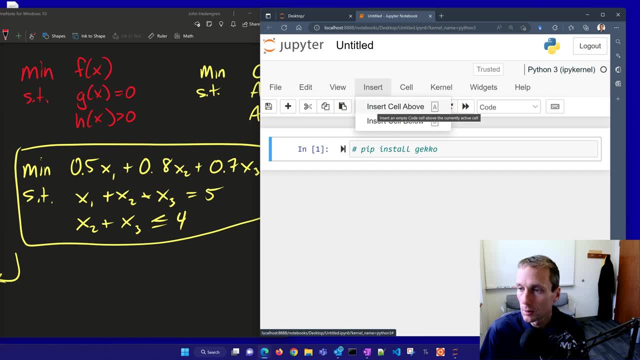 Okay, so the next thing we're going to do is just go ahead and find our model and import gecko. So I'll insert a cell So I'll say: from gecko, import gecko. and then I'll create a new model of. 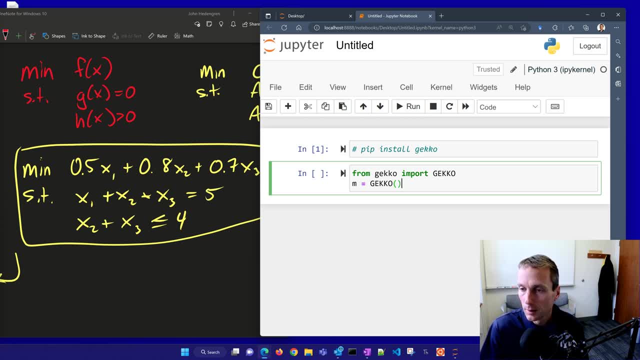 gecko. Okay, and then I'll go ahead and run that cell. So no, now I've created my model M And now I'm going to define some variables like: x one is going to be a variable, All right, x two, we'll all. 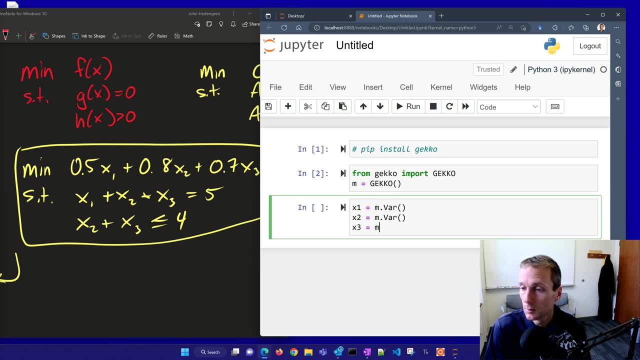 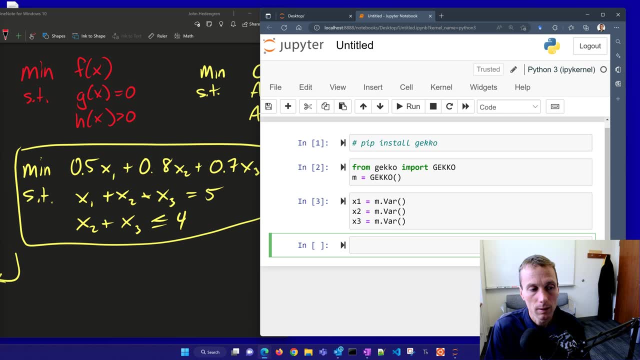 be a variable, and then x three will be a variable. All right, so I've defined my three variables, And then let's go and just define my equations now. Okay, so my first equation is: x one plus x two plus x three equals five. So don't forget the double equal sign there. And then my second: 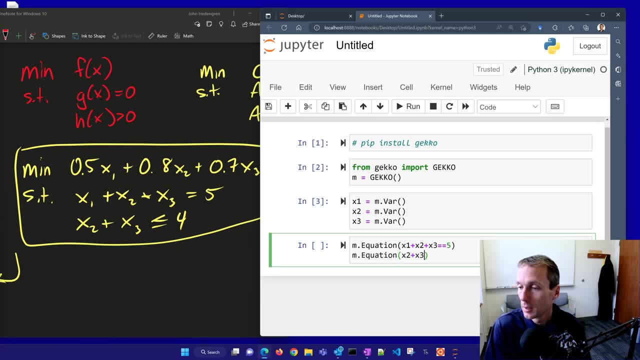 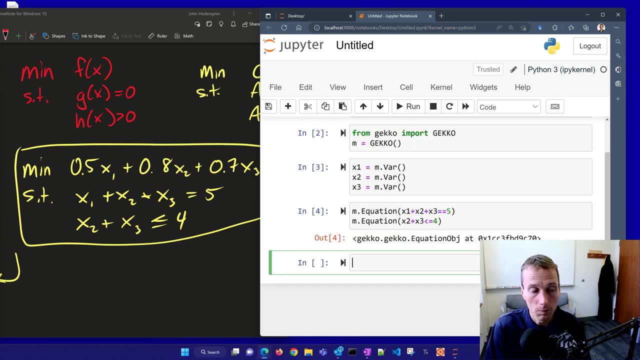 equation is going to be x two plus x three, And that's going to be less than or equal to x three Or equal to four. Okay, let's go on to our final one, which is our objective function, And we're going to try to minimize 0.5 times x one plus 0.8 times x two plus and then 0.7 times x three. 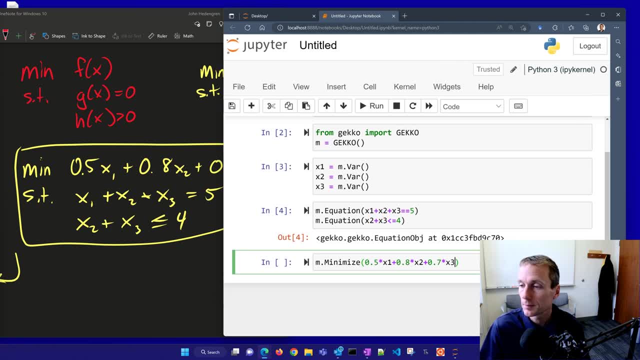 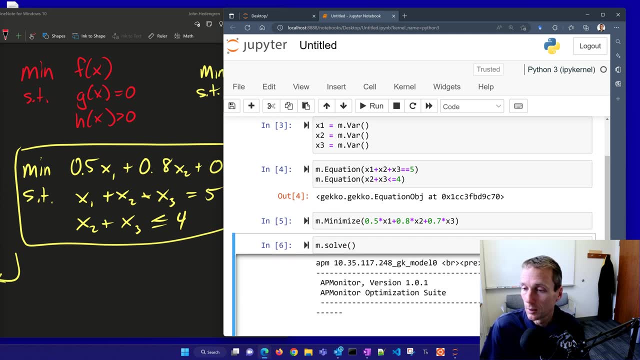 Alright, move that over just a little bit so we could see it. Okay, now we want to solve it, And this is going to put out a lot of the solver output to the screen. The main thing that you want to do when you solve this is come down here to the bottom, If it's solved it, and just look for. 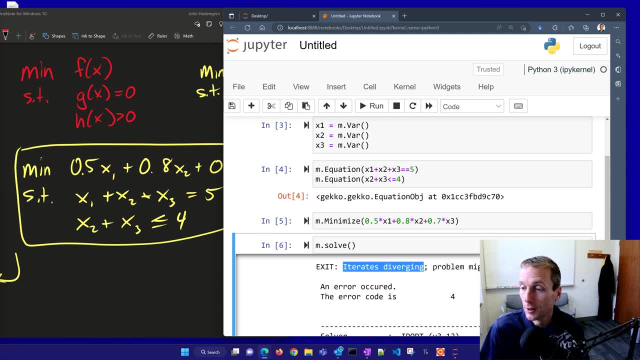 Oh, it looks like the iterates diverging. Okay, problem might be unbounded, So let's go and add some bounds to this one. Okay, so I'm going to say that lower bound equals zero and upper bound equals zero. 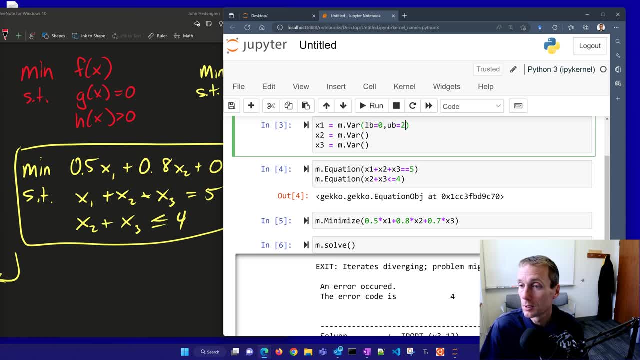 So that's where I can search for a solution. Otherwise, when I try to minimize this, all of these will go to negative infinity. Okay, or well, not all of them, but it'll try to send some of them to negative. 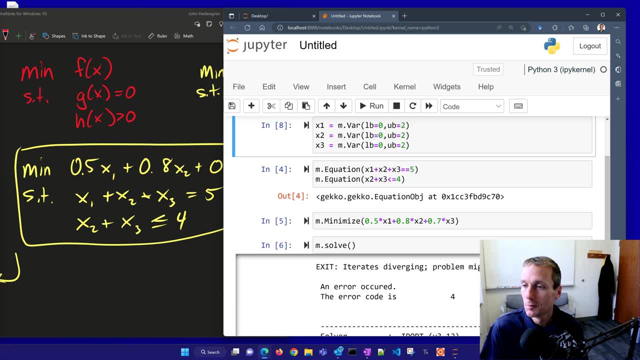 infinity. Okay, so I'll go ahead and rerun that again. Go ahead and rerun my objective function and then solve it balancedOpTimal. Okay, it looks like again I have a problem. We're gonna go ahead and just restart and run all. 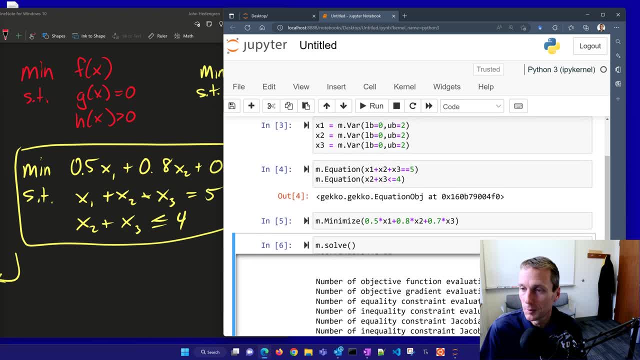 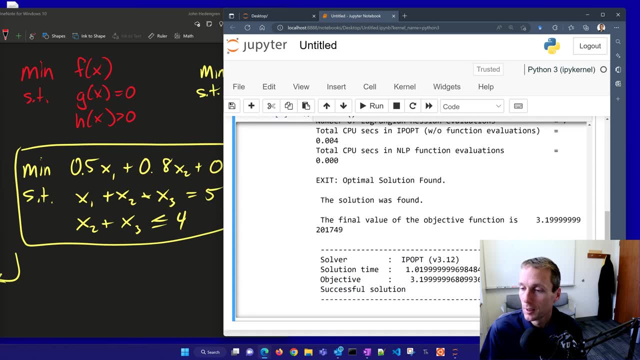 okay, there it goes. It just was holding on to some of those values from before. Okay. so when I restarted it, You could see the optimal solution is found and it gives me an objective function. So if I don't want to see all of that, It was my objective function. okay, now you might want to go and�� 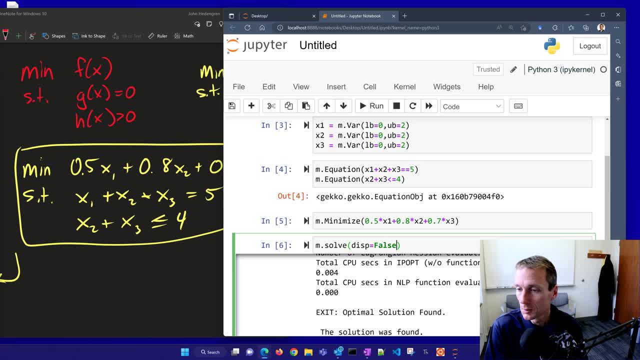 all of those values from before. okay, so when I restarted it for you could see the optimal solution is found and it output. I'll say: display equals false and then I can create a new line below that just prints the solution. okay, there's X 1 and I can put X 2 and X 3 there as. 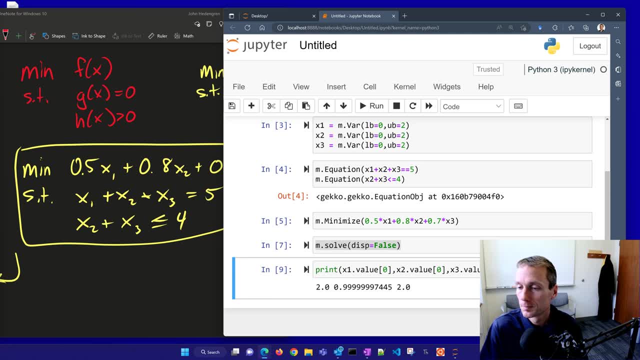 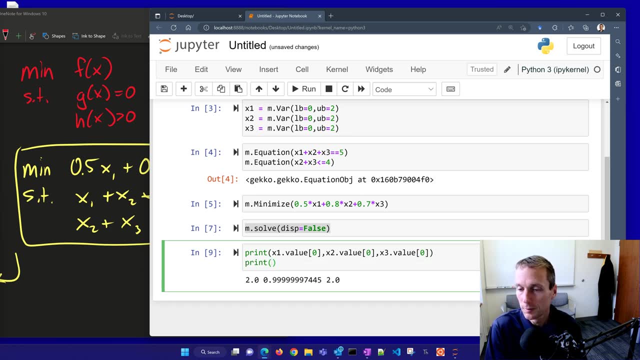 well, okay, so those are my values, and then I can also print my objective function value and that is M options- objective function value. all right, so there's my objective and then there are my three variables right there. okay, so that's a very simple problem definition using gecko. we just imported the model. 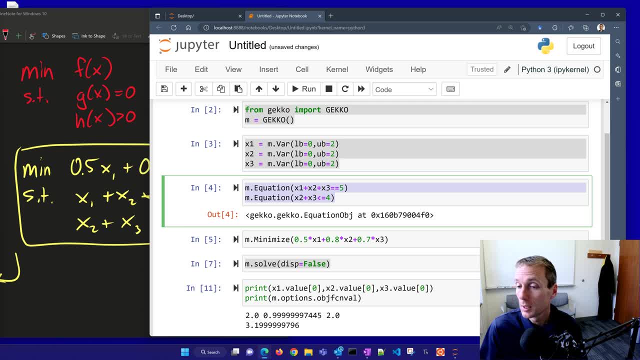 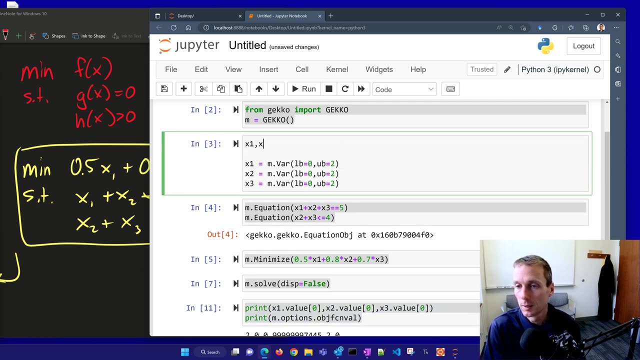 to find some variables, to find some equations. you equality or inequality, there's a minimization, I solve it and then there is my final solution. so you can also condense this down a little bit. I'll just show one way to do that. okay, I have my three X values. I can say array and. 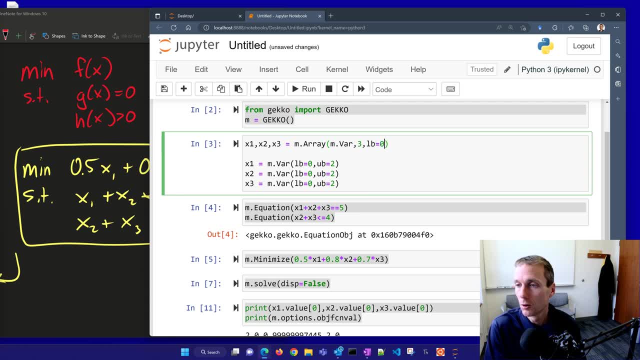 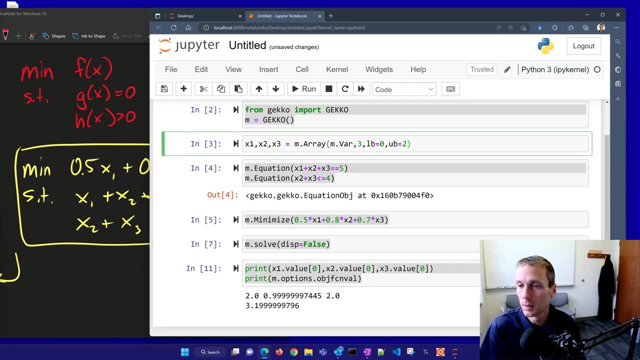 let's create three values. all of them have lower bound 0 and upper bound of 2. okay, so that's a condensed way of doing this. also, you can say equations instead and then define those as a list of equations. okay, so it simplified it down just a little bit. I'll go and throw this objective function definition in here as 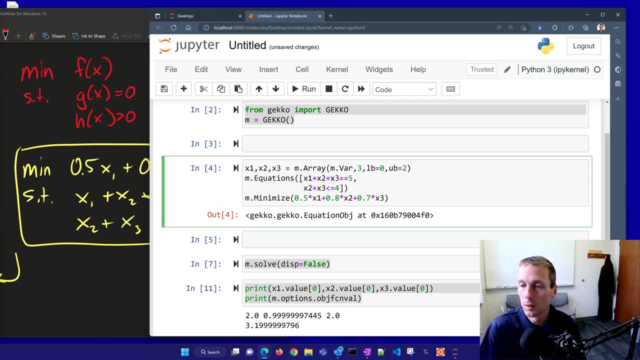 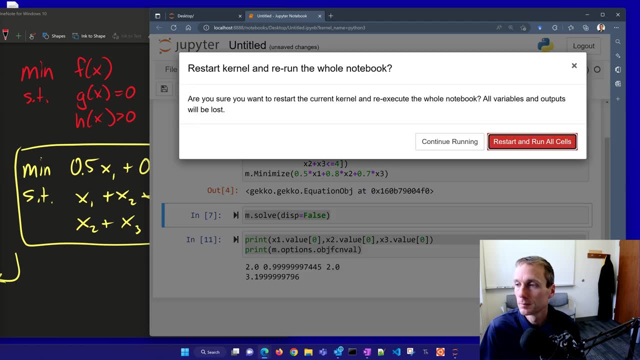 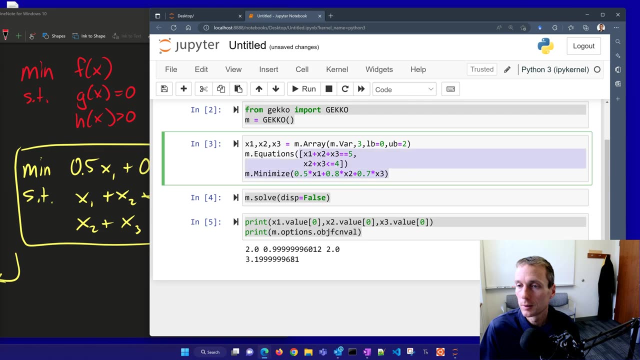 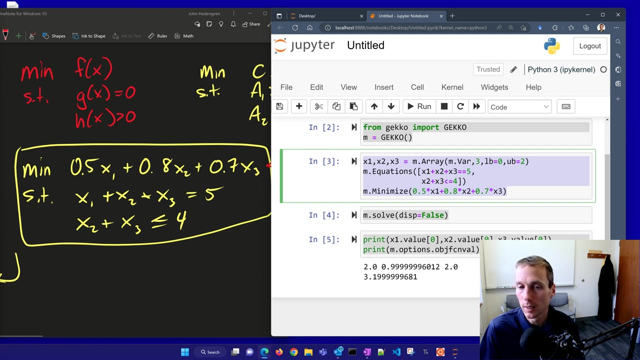 well, condense it into just one cell, okay, so I'm just restarting it and running all of it. so there's my condensed definition of the problem and you can see here it's very similar to what I had here. I just defined three variables, had my two. 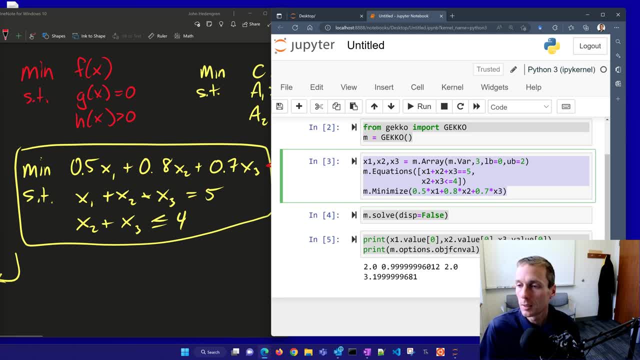 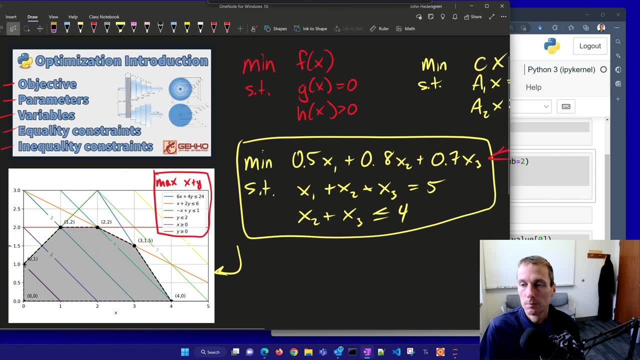 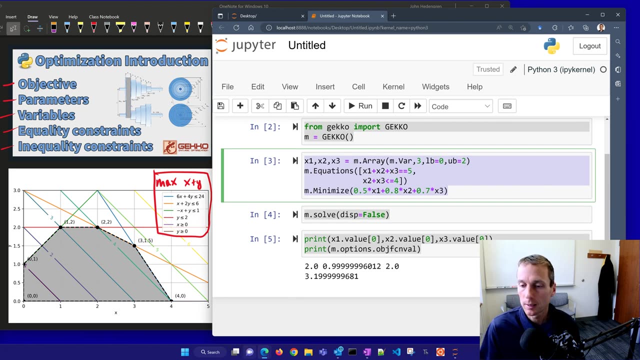 constraints as well. alright, so let's, let's solve this other one as well. we had one more that was listed here, and this is also going to be one of the exercises that will run in the next um, the next part, where we also talk about not just linear programming problems, but we also talk about some quadratic. 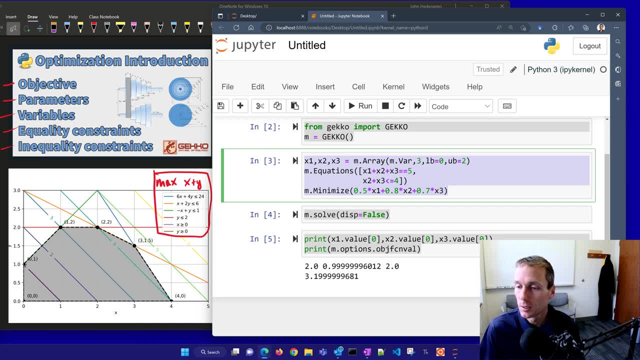 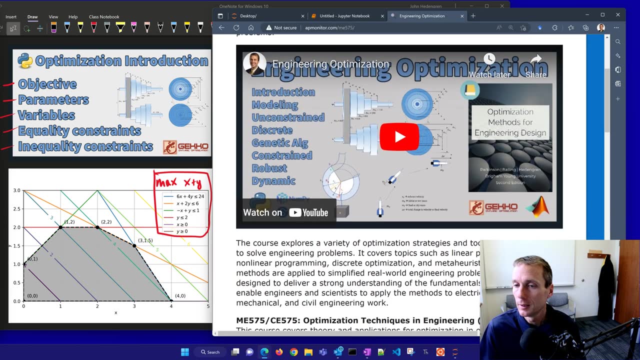 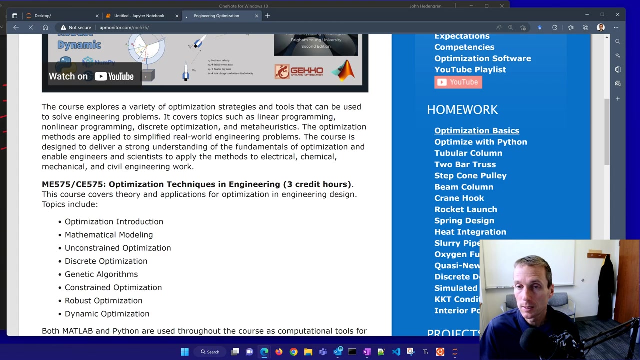 programming, non-linear programming, mixed integer and mixed integer- non-linear programming as well. so that's going to be coming up in this next. um, let's bring that up and show that to you. me 575 and here, if you just come on the side, under this is optimization basics. 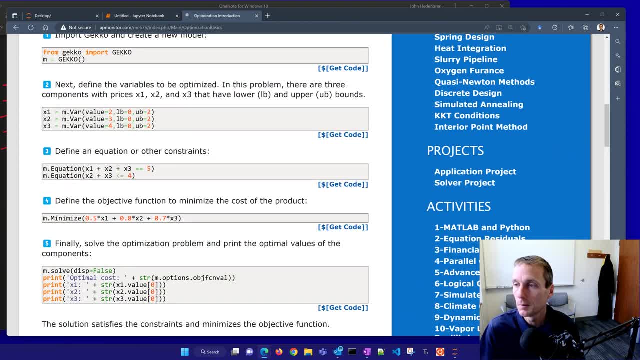 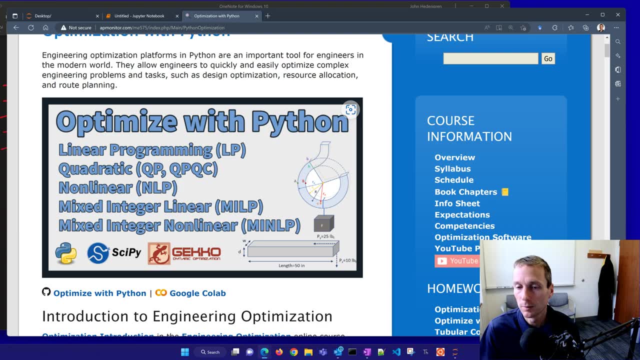 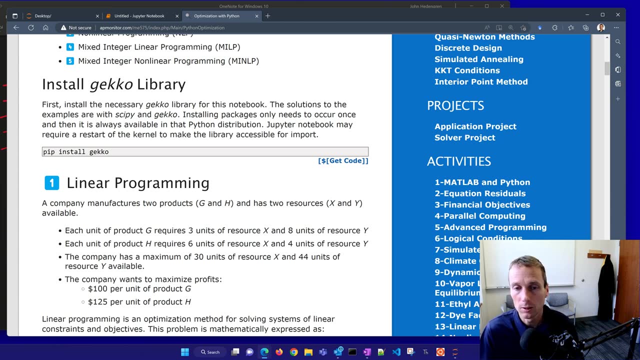 so that's what we're covering right here with this simple problem, and then the next one is going to be optimized with python and that's going to cover all of these different ones. it's going to give examples for linear quadratic, non-linear mixed integer, linear mixed integer. 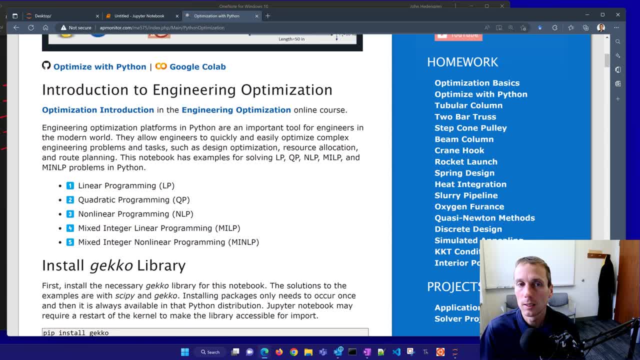 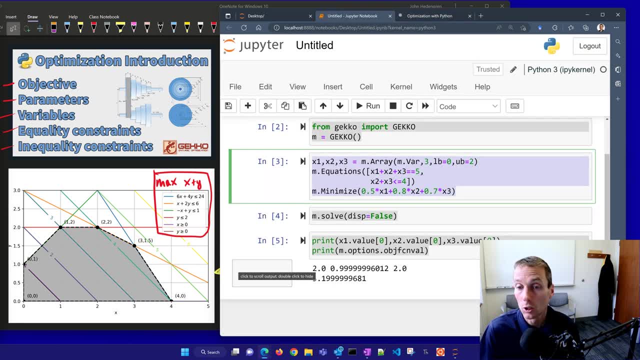 non-linear programming as well. but let's go back here and just solve this other one, so see if you can do it yourself and then pause the video and go on and check your work if you need to. so try to solve this one over here on the left with this minimization problem. 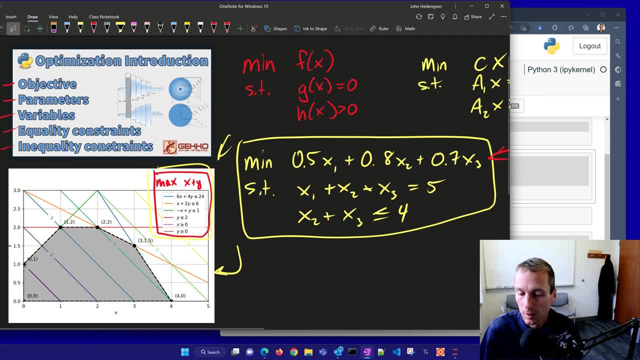 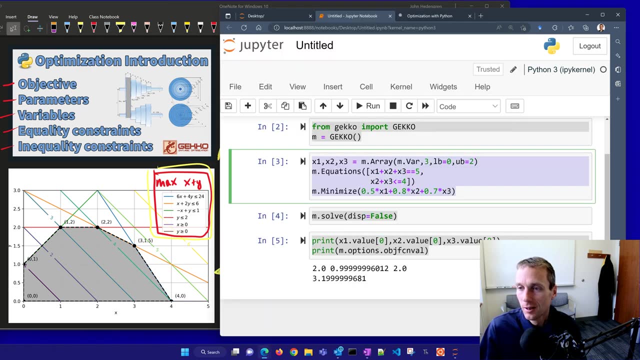 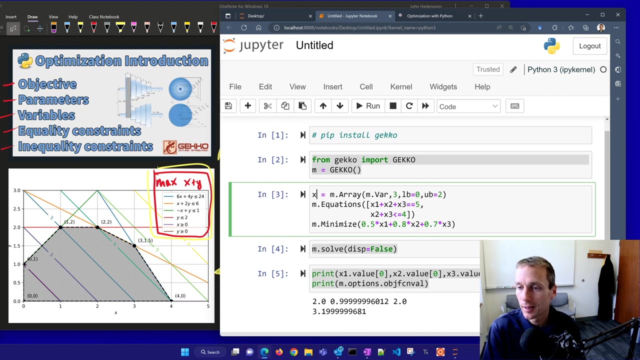 that you see right here, actually it's. i guess it's a maximization problem. okay, we're maximizing x plus y, okay, so go ahead and pause and try it yourself, all right? well, let's uh, go through this together. we're going to first of all just say that we have x and y, and we only have two values there. 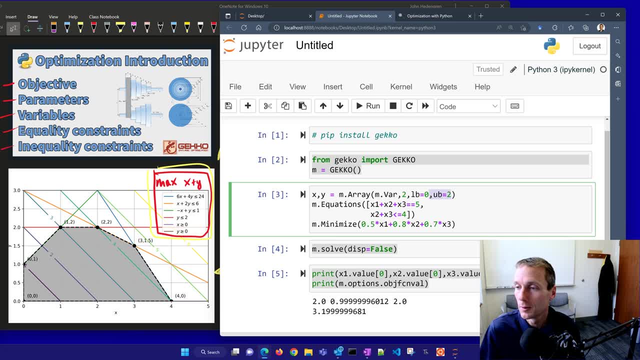 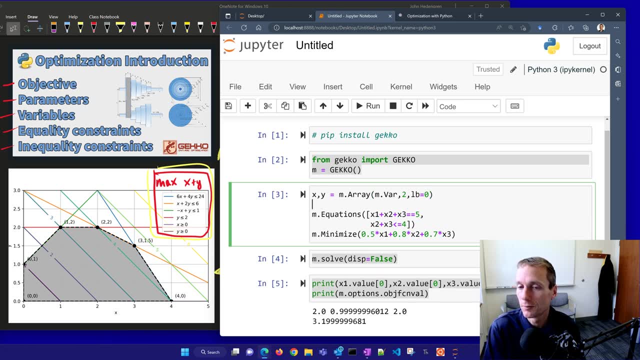 um, and then we're also going to say that we have a lower bound of zero, but y is going to have an upper bound as well. we'll just change that for the y value. okay, so y is upper, is going to be equal to two. okay, and x doesn't have an upper bound. our equations are going to be six, six times x plus four. 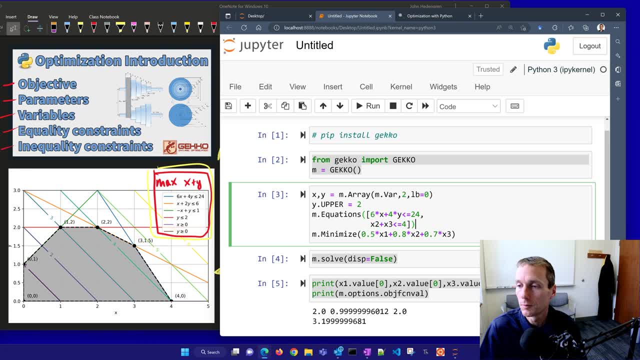 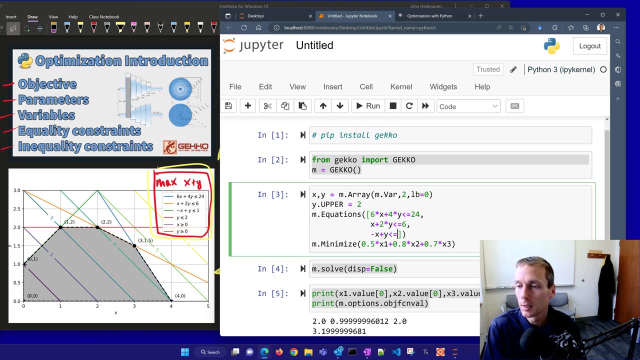 times y is less than or equal to 24.. our second one is going to be: x plus two times y is less than or equal to six, and then let's just create a new one here: minus x plus y is less than or equal to one, and then i already have the other ones listed as simple bounds instead. now let's go ahead and 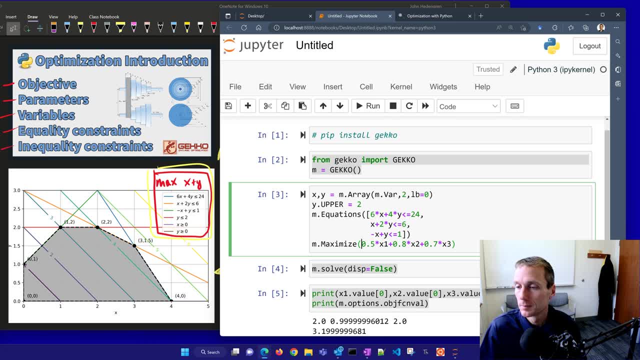 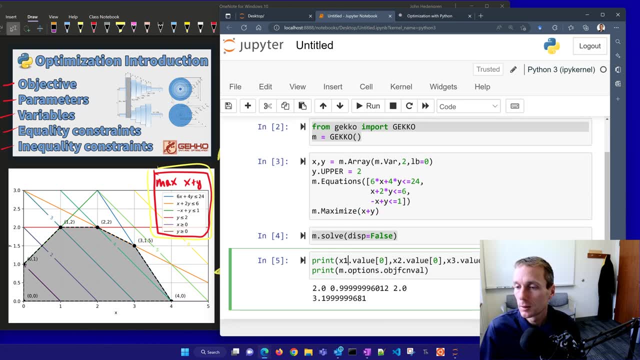 just change this to maximize x plus y, okay, and then i'll just change this to x value and y value, and then i can go ahead and delete this x3. okay. there we go, okay. so i'll just restart and run all the cells and let's just see. 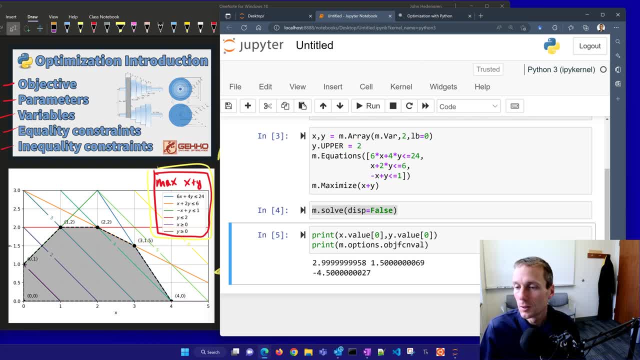 the value of the value of x plus y that it gives me. so it came up with something fairly close to three. it's not exact. these are numerical solutions. and then you can see the y value of 1.5 and then the objective function, because i'm maximizing it. you just put a negative in here because it converts it to a minimization. 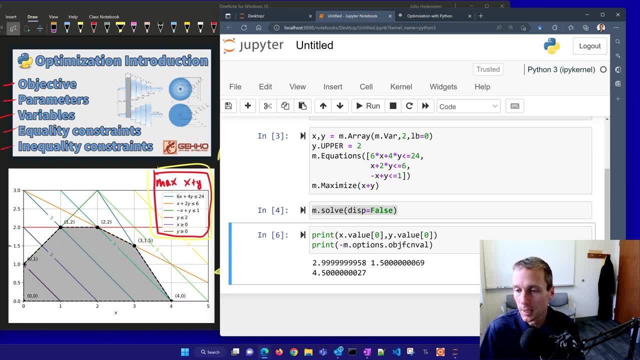 problem when it solves it, and it does that by just multiplying by negative one. so let's just look at our chart over here on the left just to see how it did, and we can see that it's not exactly the same function as the previous one. so, again, nothing special to it. let's go ahead and 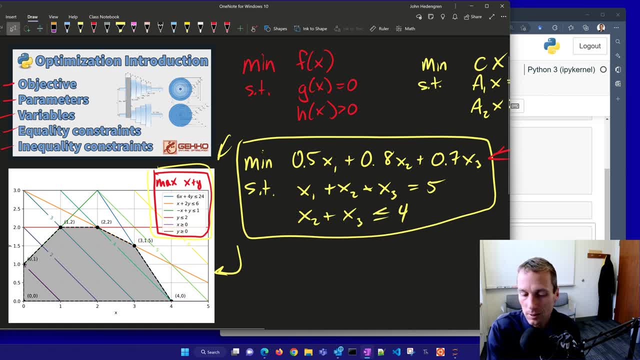 write through the area line. here we can usually draw the second. and finally, i'd comment on that that the positive function is the one in the denominator. and right there we have today, and we'll sort ofера this a little bit just easier, a little bit sort of. 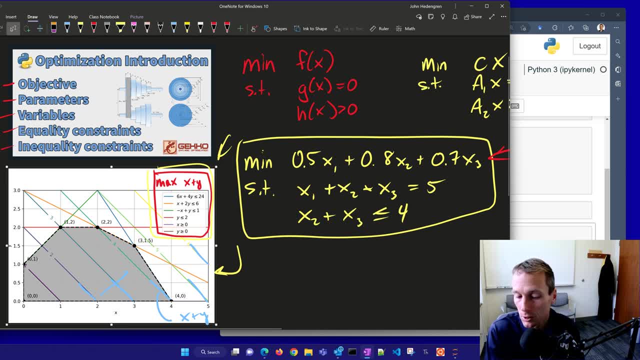 do another campo example, okay, and then let's just render this so picture. so if we We know in linear programming that the solution is going to be at one of these vertices, the intersection of the constraints, And so like in the simplex method, you just go through and successively evaluate. 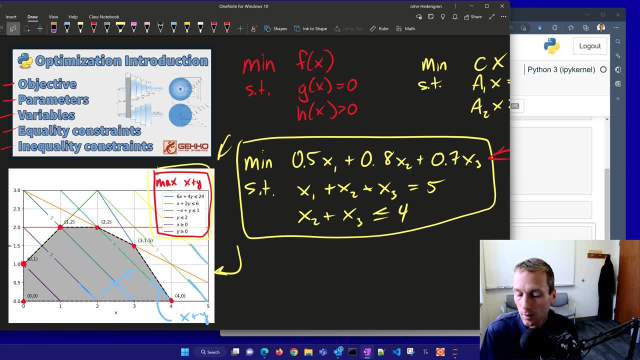 just these intersections to find a solution. Well, we can see that. this one right here, the objective is 4.. This one down here, the objective is also 4.. But right here, the objective is 4.5.. So that's going to be our best solution. 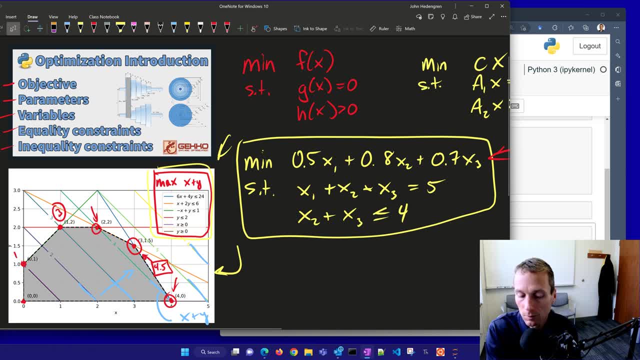 This one over here is 3.. This one over here is 1. And then this one is 0. So if we're trying to maximize between all these different objective options, the best one is going to be right here, And we can see that with our solution as well. 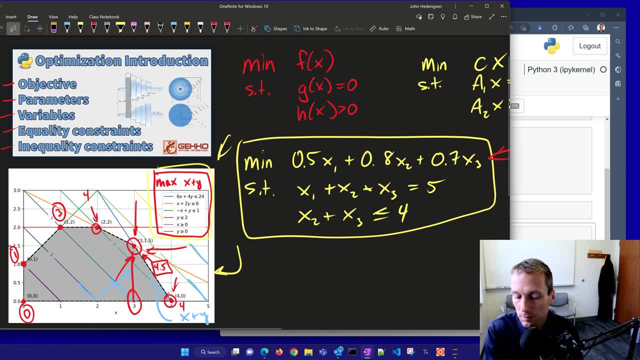 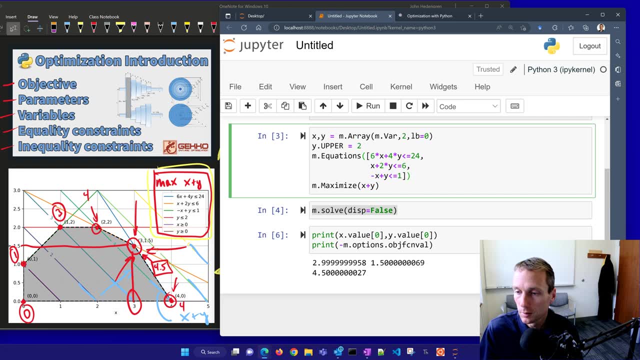 We got. We got an x value of 3 and a y value of 1.5.. So it was able to find the best solution out of all those potential ones with an interior point solver. So the other thing you'll see with this, as we'll go later on. 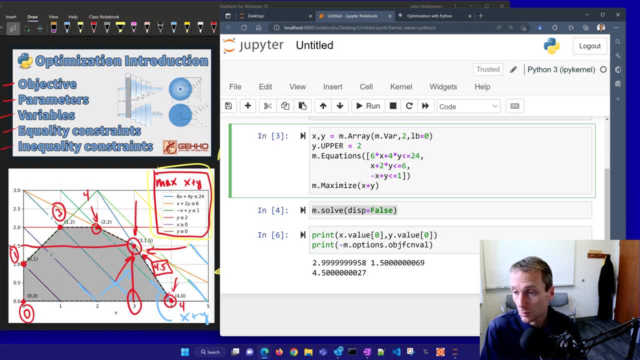 is. you can also put in nonlinear or quadratic terms as well. So I could have, I could have something like this, And if I restart and run all then you'll see it comes up with a different solution. Okay, When I have a different objective function that might be nonlinear instead. 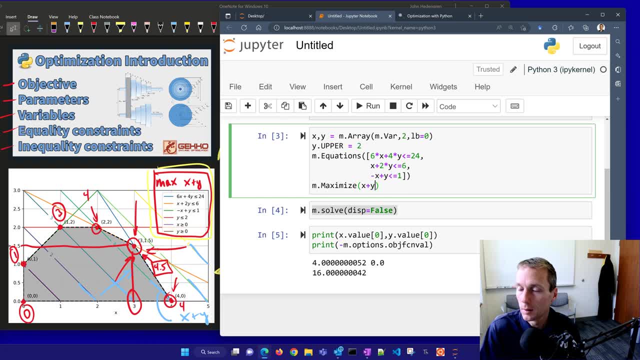 Okay, But for this one that was just x plus y, we have a solution right up here, Okay. Well, I hope you've enjoyed this optimization introduction. We're going to go on to our next one, as I mentioned, and solve not just linear programming.